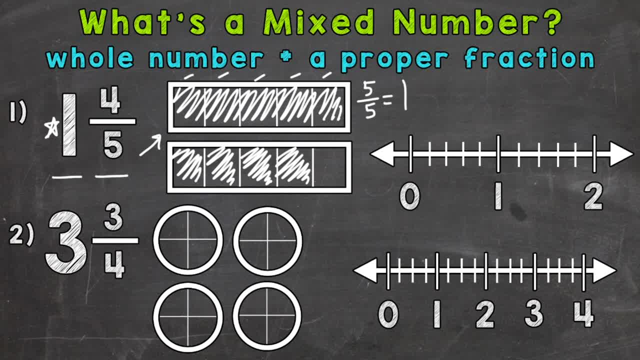 two wholes. You'll notice that we almost have two wholes there, but not quite, So let's fill in one whole rectangle. I've filled that in down again. We'll fill in a multiple, then a multiple year, Don't you? you, f, u and f. 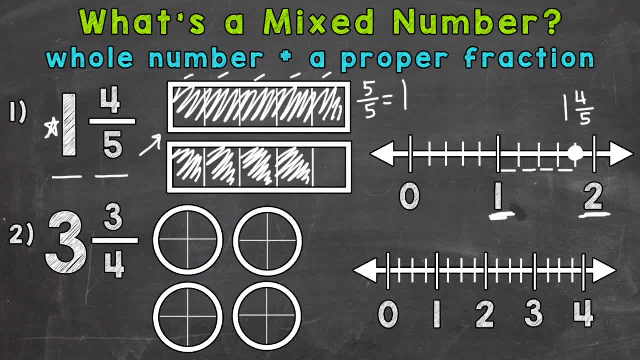 Now I do want to mention that mixed numbers can also be expressed as improper fractions, And an improper fraction is a fraction where the top number, the numerator, is greater than the bottom number, the denominator. Mixed numbers and improper fractions are equivalent. 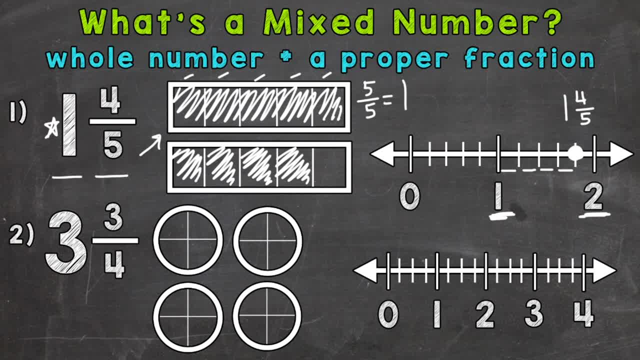 They can represent the same value. it's just two different ways to write out that value. So, for example, number 1, 1 and 4 fifths is actually equivalent to 9 fifths. So we can take a look at our model and we have 1,, 2,, 3,, 4, 5, 6,, 7,, 8, 9 fifths filled. 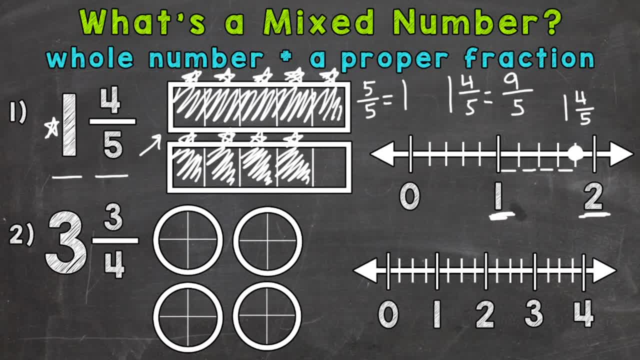 in, So we can see that 1 and 4 fifths is equivalent to 9 fifths. Now there's another way to write this. There's another way to convert between mixed numbers and improper fractions, but that's a topic for another video. 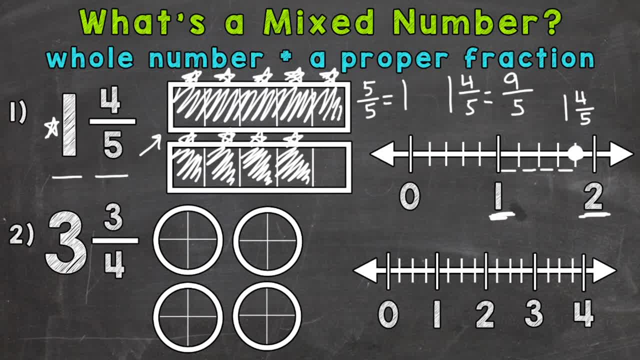 I'll drop other links to improper fractions and other fraction topics down in the description. So let's move on to number 2, where we have 3 and 3 fourths, So again a mixed number. we have a whole number plus a proper fraction. 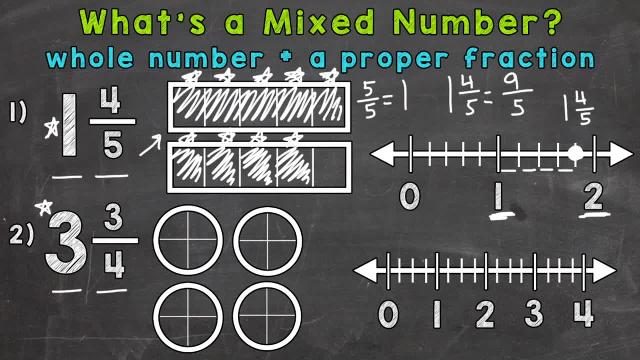 So let's model this first, and we first need to fill in 3 holes. So we'll use circles this time. So 3 whole circles to represent the whole number And then the proper fraction portion. we have 3 fourths. 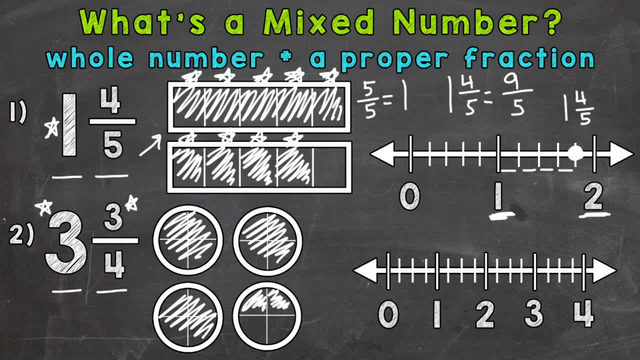 So 1 fourth, 2 fourths and 3 fourths. So that would be 3 and 3 fourths, modeled there using whole circles, And then our proper fraction, portion 3 fourths. So over to the number line where we need to start with the 3..